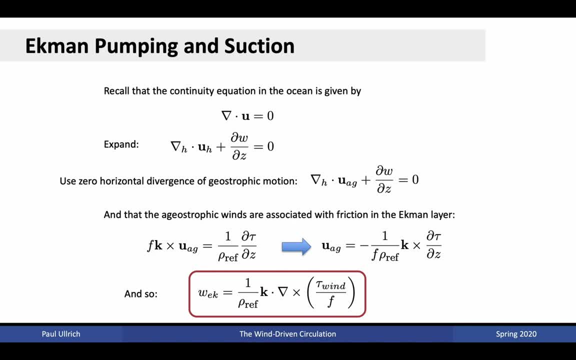 this reveals that this divergence of the horizontal velocity is in fact the horizontal divergence of the a-geostrophic wind, And so that allows us to simplify this equation somewhat. We also use that the a-geostrophic winds are associated with friction. 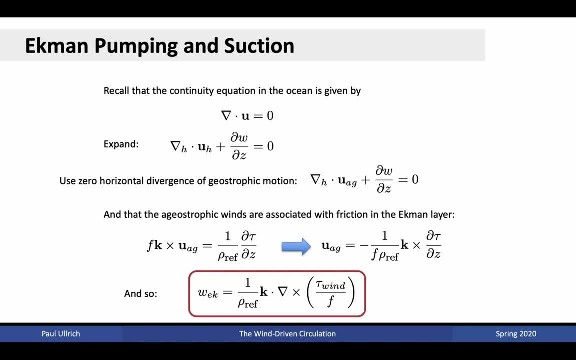 and the Ekman layer. That is from last time we had an equation that looked like: f k cross, u? a-g is equal to one over rho reference times, the vertical derivative of the stress. We can transform this into an equation for u? a-g by doing k cross on both sides. The result is u? a-g equals negative. 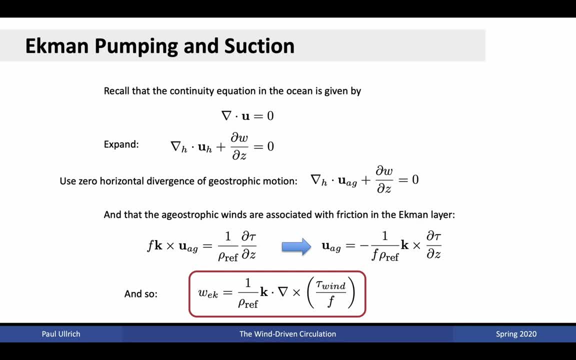 one over f? rho reference times. k cross the vertical derivative of the stress, And so we obtain that the vertical velocity induced by the Ekman layer is given by one over rho reference times, the vertical derivative of the stress. Here we have a total reference k dot curl of the wind stress divided by f. 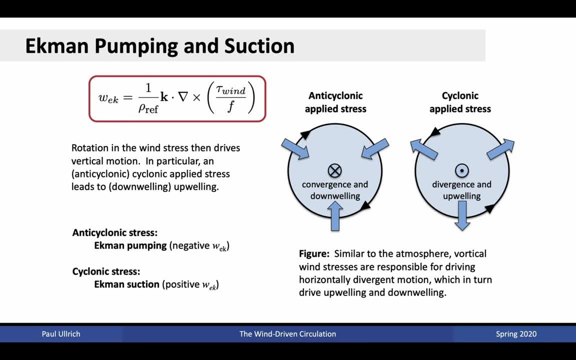 Okay, what does this equation imply? Well, recall, this k dot curl term has popped up before in our discussion of vorticity. back in atmospheric dynamics, If we have a flow that is counter, that is rotating counterclockwise, then typically that's associated with a positive vorticity. 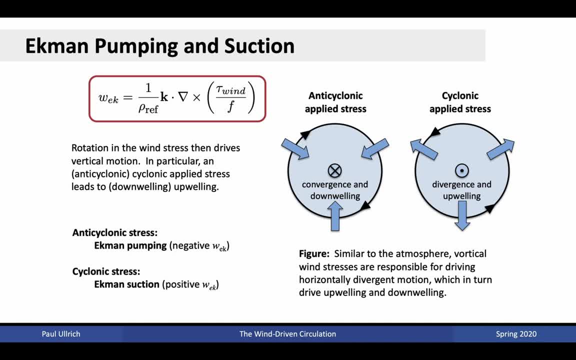 If it's rotating clockwise, that's associated with a negative vorticity. Here we also have a Coriolis term that comes into the mix: the 1 over f term. This implies that whenever we have an anticyclonic applied stress, that is, in the northern hemisphere, we have a clockwise applied 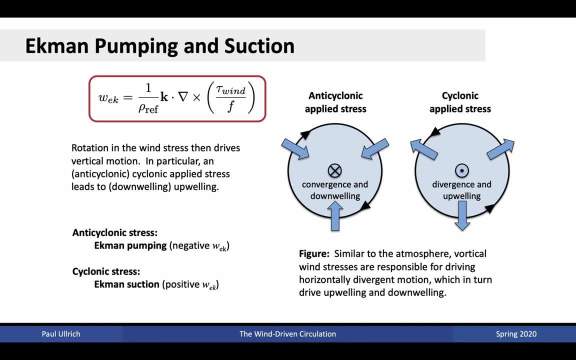 stress and in the southern hemisphere a counterclockwise applied stress, this k dot curl term will be negative. On the other hand, if we have in the northern hemisphere counterclockwise rotation or in the southern hemisphere counterclockwise rotation, then this k dot curl 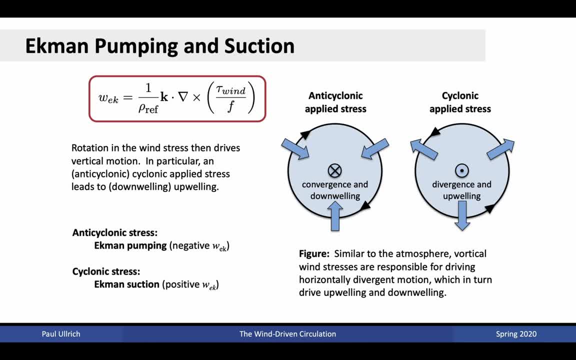 term will be positive. So how does that work out for the ocean then? If we have an anticyclonic applied stress because of the wind field, we then have convergent motion, which is then responsible for driving a negative vertical velocity In the ocean. this is known as downwelling. 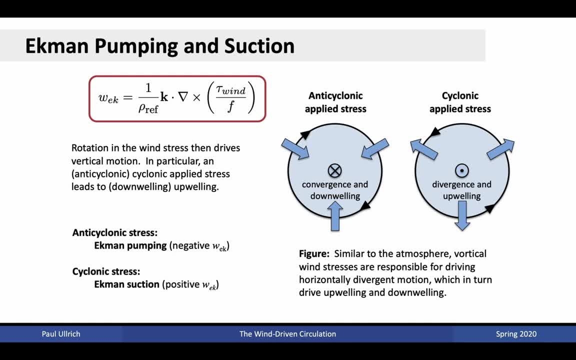 That is, we have ocean waters at the surface that are being pushed downwards. So this anticyclonic stress then induces convergence and downwelling. in much the same way, a local surface low in the atmosphere would also induce convergence. On the other hand, if we have a cyclonic applied stress, again this is a 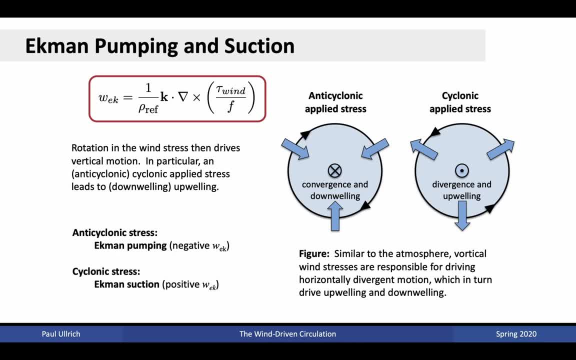 counterclockwise rotation in the northern hemisphere. then we have divergent motion and upwelling. In the case of upwelling, ocean waters are pulled from downwelling and upwelling. So this is a counterclockwise rotation in the northern hemisphere. 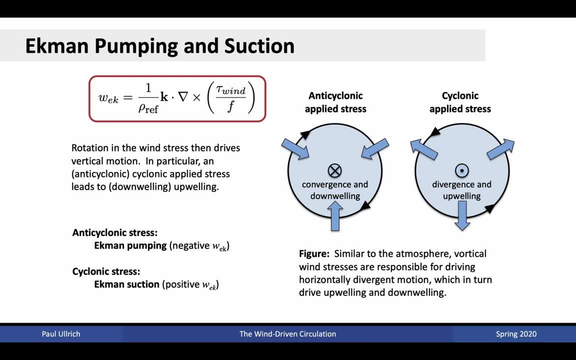 If we have an anticyclonic applied stress, again this is known as downwelling. This is known as downwelling. So this anticyclonic applied stress then induces convergence and downwelling. So this anticyclonic applied stress then induces convergence and upwelling. 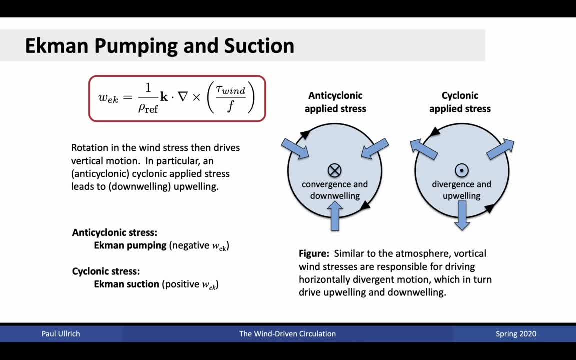 So, in summary, anticyclonic stress induces Ekman pumping, That is, negative vertical velocities associated with pumping near-surface waters to depth. Cyclonic stresses are associated with Ekman suction, That is, sucking waters up from depth in order to replace waters that 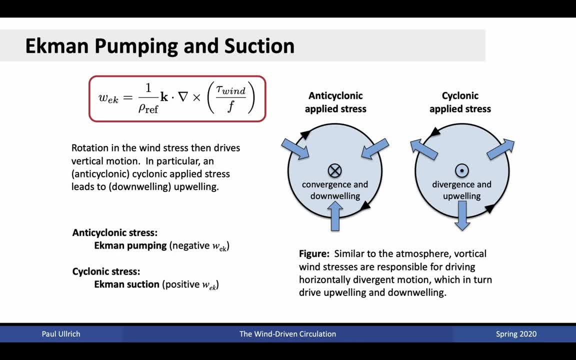 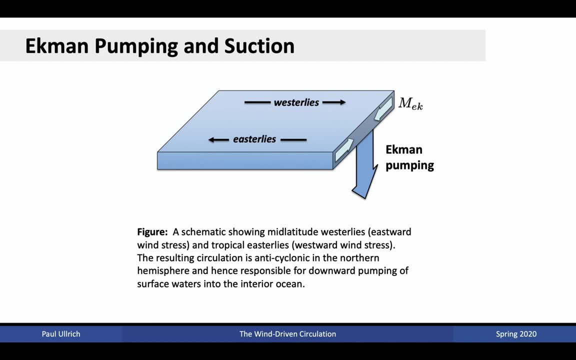 diverge at the surface. Anticyclonic applied stresses are then analogous to surface low lows in the atmosphere, and cyclonic applied stresses are analogous to surface highs. Okay, how does this apply, then, to the ocean gyres? Well, in the northern hemisphere, the subtropical gyre is associated with easterlies to the. 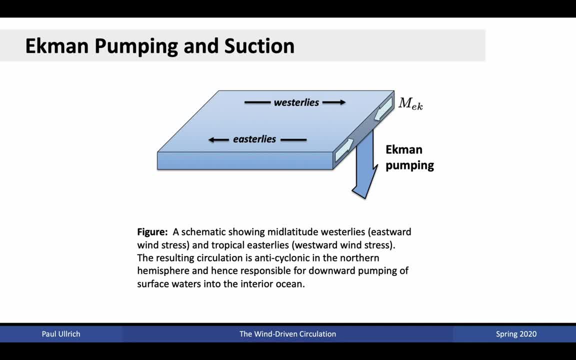 south and westerlies to the north. This is then an anticyclonic rotation. Recall that anticyclonic rotation is associated with Ekman pumping, so the presence of these ocean gyres then result in water being pumped from the near surface to depth. 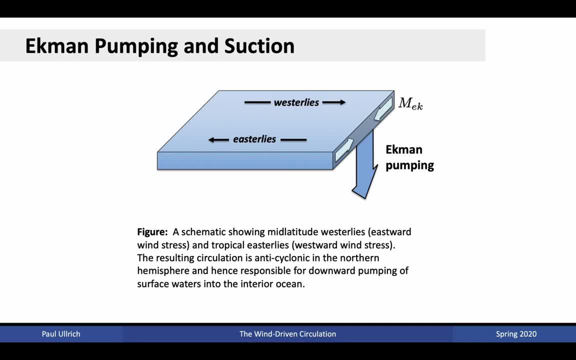 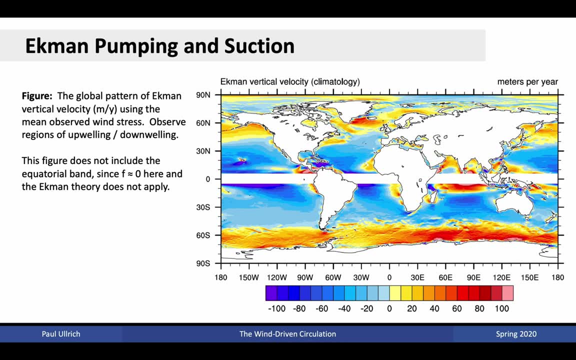 That is, we have a vertical velocity, a negative vertical velocity, which is induced because of the anticyclonic rotation in this gyre. We can look at a plot of the global pattern of Ekman: vertical velocity as a function of location. 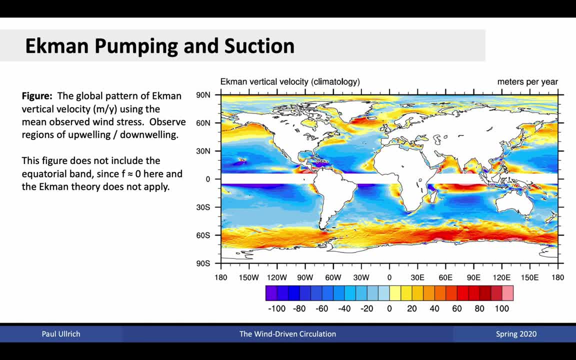 In the regions where we have anticyclonic ocean currents, namely the subtropical gyres, we see negative vertical velocities. These vertical velocities effectively cause the shallow water lines and 되면 coming together. There is, then, a particular role in this particular rainsite that needs to be carried. 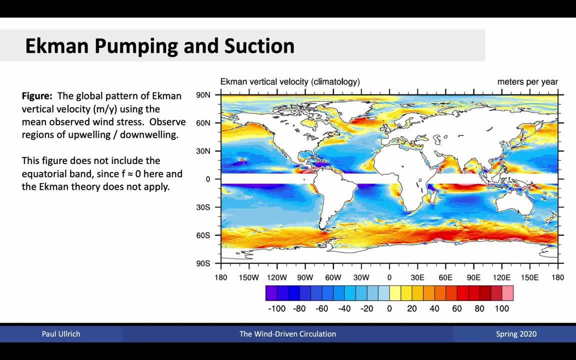 by a spout between two depressions and two basins and why theussian counts. Specific letters are a good example of privateificators. – ev法ис, Platz 2 – z-a Formats: hands stunt up is very small. The units of this, the units shown in this map, are actually. 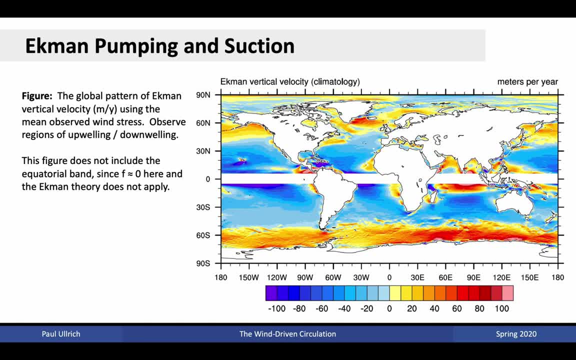 meters per year, so it's not a very significant amount, and this is reflective of the fact that ocean currents do operate very slowly. The ocean does operate on much longer time scales than the atmosphere, so this is perhaps not surprising Over very long time scales. nonetheless, the Ekman 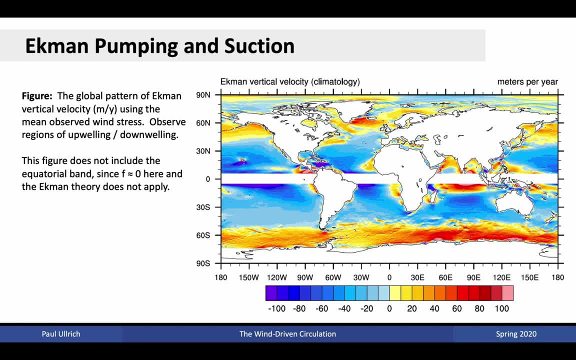 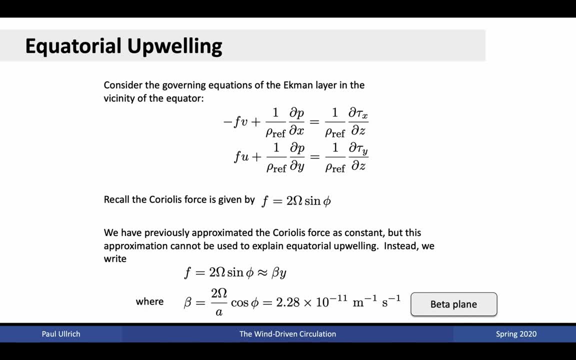 velocities are important for changing the vertical structure of the ocean. This theory cannot be used to explain what occurs in the equatorial regions, because in these regions the Coriolis parameter is approximately zero. Recall that this parameter enters into the denominator of the previous expression. 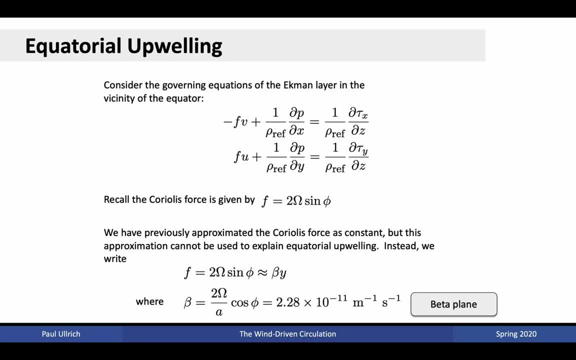 for the Ekman induced vertical velocity. So we're going to have to modify the theory somewhat. Instead of assuming a constant Coriolis parameter, we'll instead assume a beta plane. Under the beta plane approximation we have a linearly varying Coriolis parameter with distance away from the equator, Namely f is. 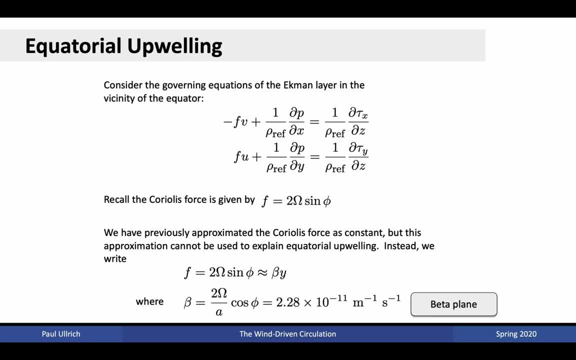 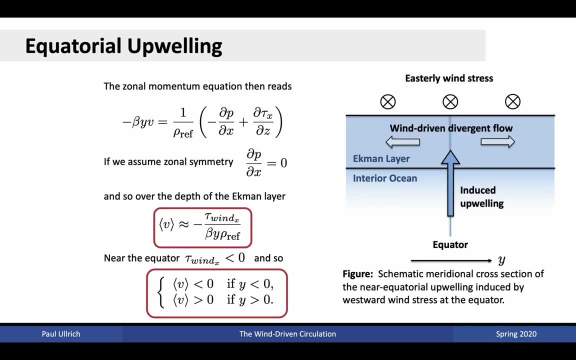 approximated as beta y, where y is the distance away from the equator and beta is a constant coefficient. If we plug this now into the zonal momentum equation, we get the equation above. If we now assume zonal symmetry, namely that di p, di x is equal to zero, as is a reasonable approximation in the 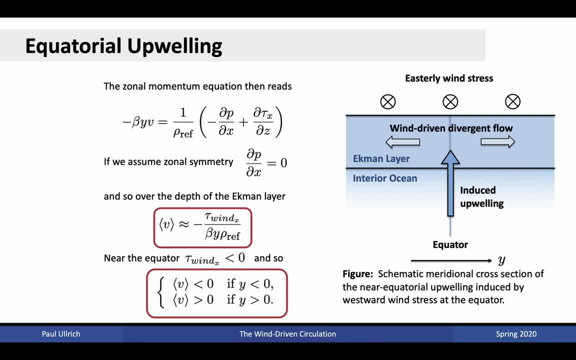 equatorial regions. We then obtain that, over the depth of the Ekman layer, that the meridional velocity induced by the wind stress is going to be given by negative tau wind x divided by beta y row reference. This expression is nonetheless not valid when. 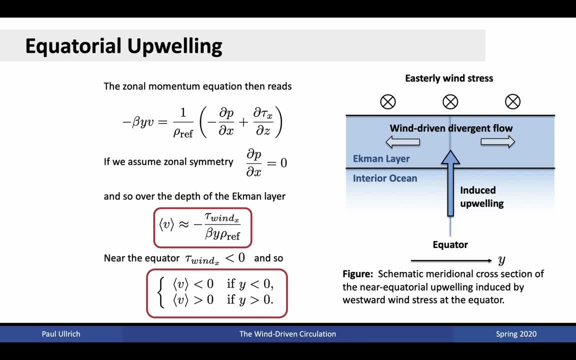 y is equal to zero, but when we move towards positive or negative values of y, it does indicate that there is a meridianally induced current velocity because of the presence of a zonal wind stress, Namely north of the equator, where y is positive. 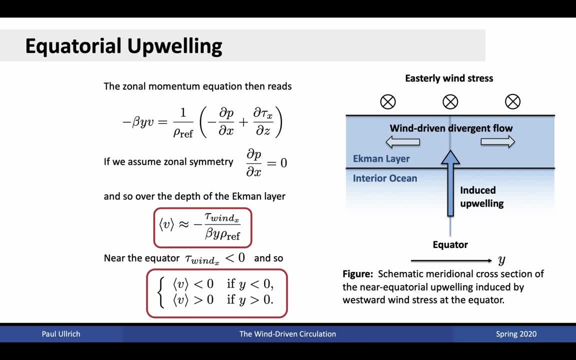 we have that the meridional velocity is proportional to negative tau wind x. Now which direction is the wind blowing in in these regions? From what we know before about the general circulation of the atmosphere, recall that the wind is blowing from east to west. 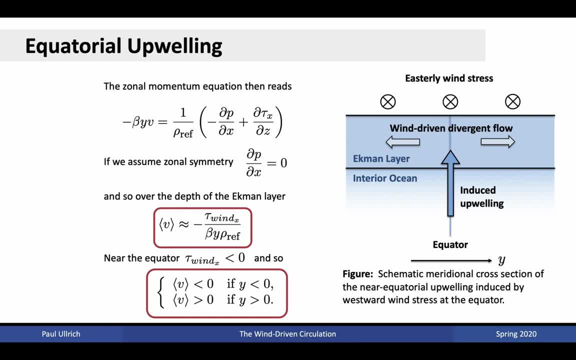 Namely it's an easterly wind stress, So this quantity tau wind x is negative. What that means, then, is that north of the equator we must have that the meridional velocity is positive, and south of the equator we have that the meridional velocity is negative. 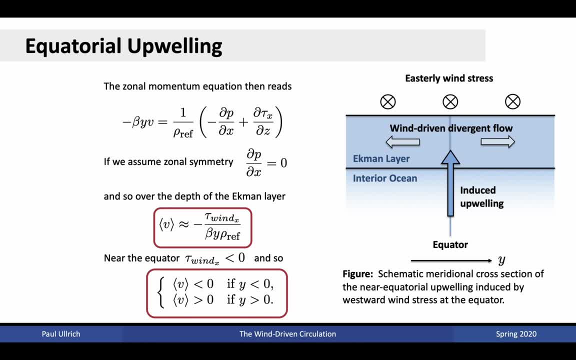 So the presence of this easterly wind stress in the equatorial region then drives a divergent flow, That is, water is pushed poleward away from the equator. In order for this to satisfy conservation of mass, we must then have that there is an induced 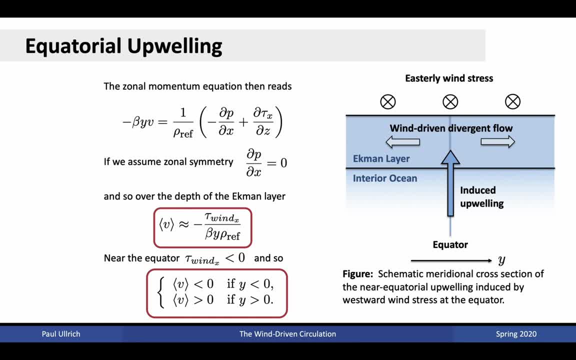 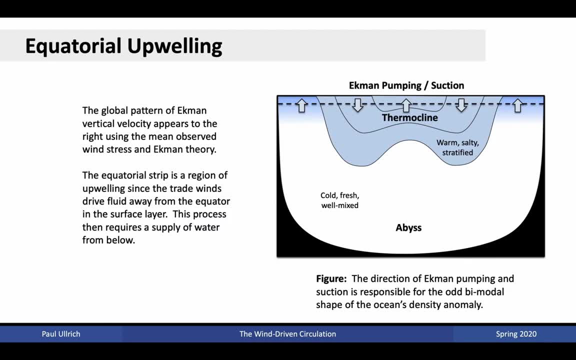 reduced upwelling in this region, where water is pulled from depth in order to replace the water that is being that is diverging from the equator. So now that we know that in the equatorial regions we have upwelling, or Ekman suction. 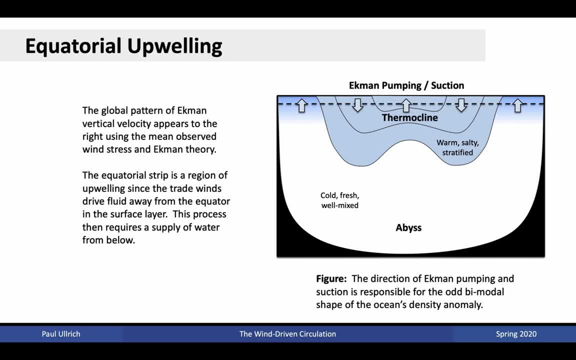 in the subtropics we have downwelling or Ekman pumping, and in the polar regions we have upwelling or Ekman suction. we then have a better understanding of why the latitudinal vertical cross-section of the ocean looks the way that it does. 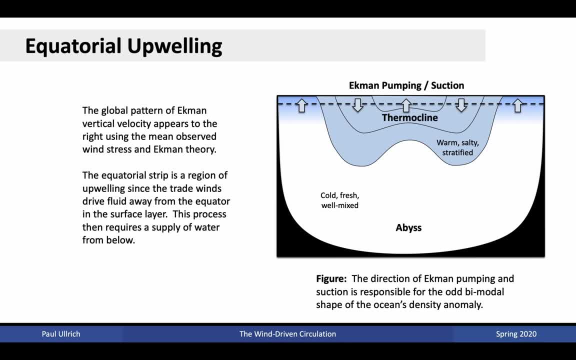 Specifically, these warmer near-surface waters are pumped to depth because of Ekman pumping in the subtropics, and the colder deep ocean waters are pulled up because of the presence of Ekman suction at the equator. Consequently, we have this bimodal shape associated with thermocline. 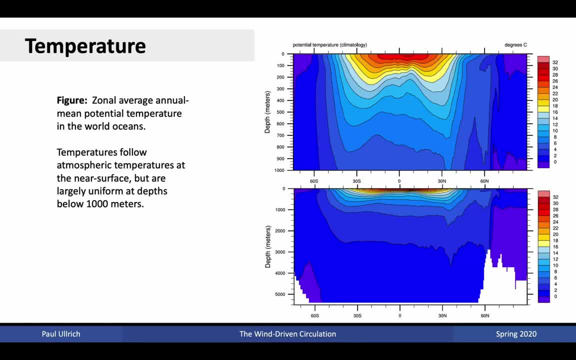